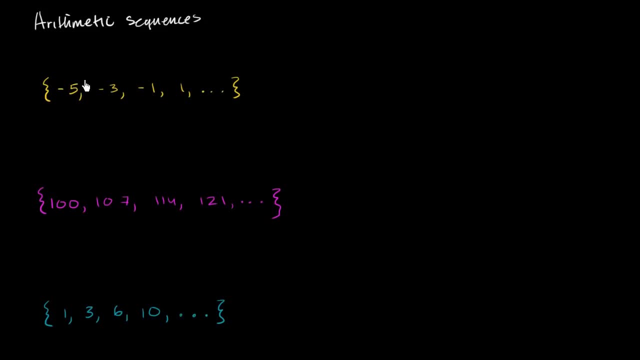 Well, let's look at this first one right over here. To go from negative 5 to negative 3, we had to add 2. Then to go from negative 3 to negative 1, you have to add 2. Then to go from negative 1 to negative 2, you had to add 1 to 1. 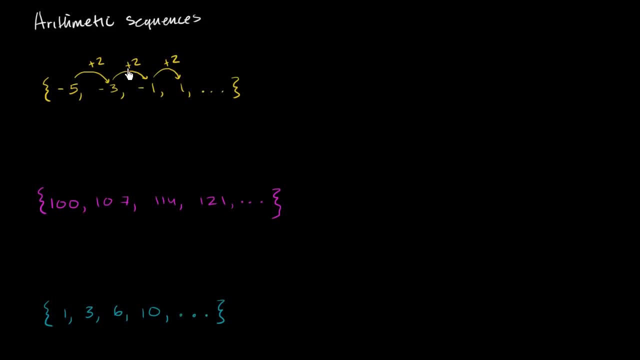 You had to add 2. So this is clearly an arithmetic sequence. 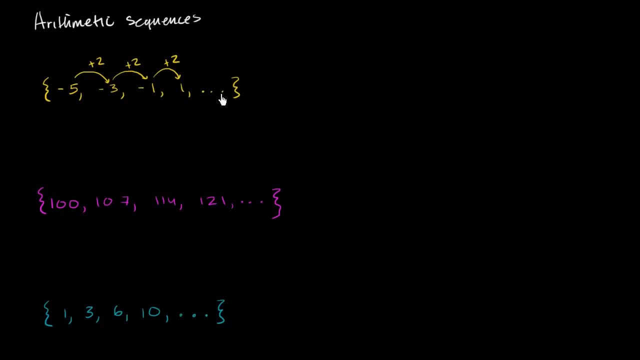 We're adding the same amount every time. And there's several ways that we could define the sequence. We could say it's a sub n. And you don't always have to use k. This time I'll use n to denote our index. From n equals 1 to infinity with. And there's two ways we could define it. We could either define it explicitly or we could define it recursively. 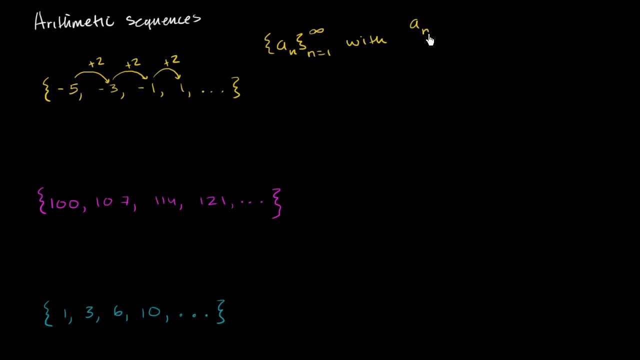 So if we wanted to define it explicitly, we could write a sub n is equal to 1. Is equal to whatever the first term is. In this case, our first term is negative 5. It's equal to negative 5 plus we're going to add 2 one less times than the term we're at. So for the second term, we add 2 once. 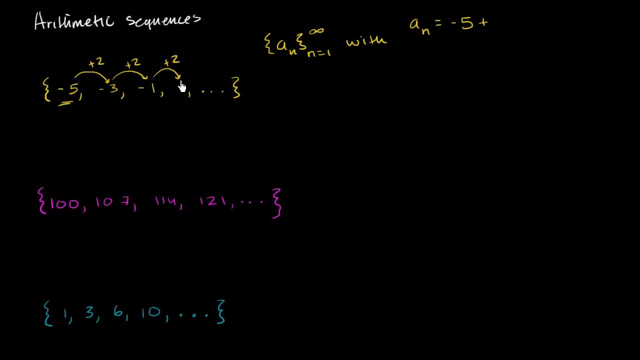 For the third term, we add 2 twice. For the fourth term, we added from our base term, we added 2 three times. So we're going to add 2. We're going to add positive 2. 1 less than the index that we're looking at. n minus 2. Minus 1 times. So this is an explicit definition of this arithmetic sequence. 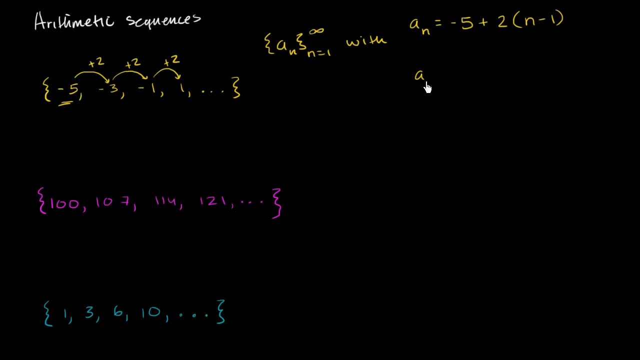 If I wanted to write it recursively, I could say a sub 1 is equal to negative 5. And then each successive term for a sub 2 and greater. So I could say a sub n is equal to a sub n minus 1 plus 3. Each term is equal to the previous term plus 2. Not 3. Plus 2. So this is for. For n greater than or equal to 2. 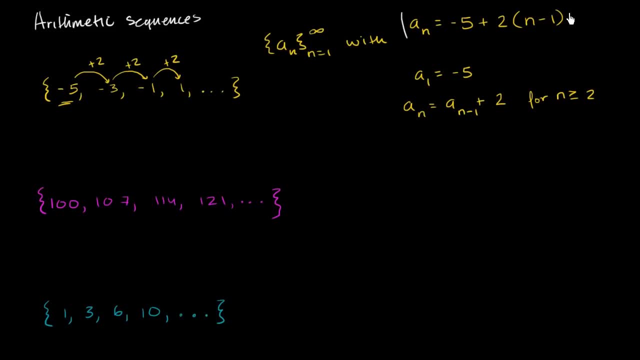 So either of these are completely legitimate ways of defining the arithmetic sequence that we have here. 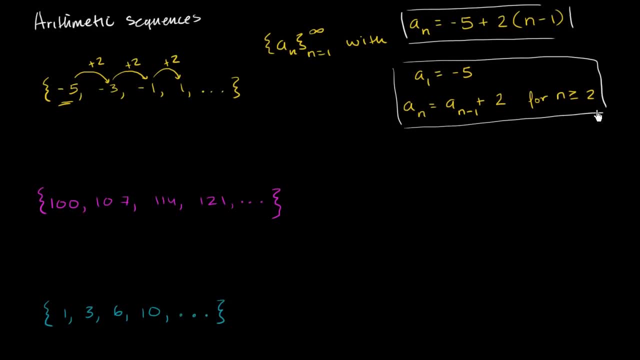 We could either define it explicitly or we could define it recursively. 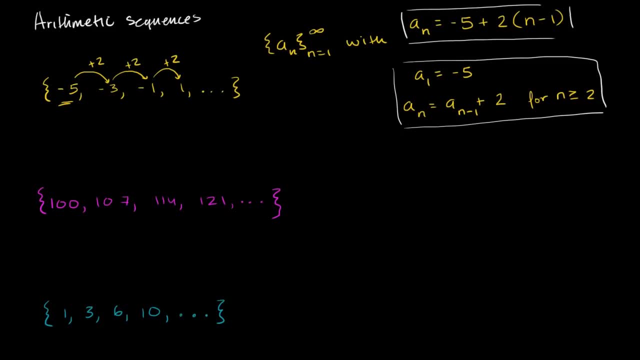 Now let's look at this sequence. Is this one arithmetic? Well, we're going from 100. We add 7. 107 to 114, we're adding 7. 114 to 121. 121. 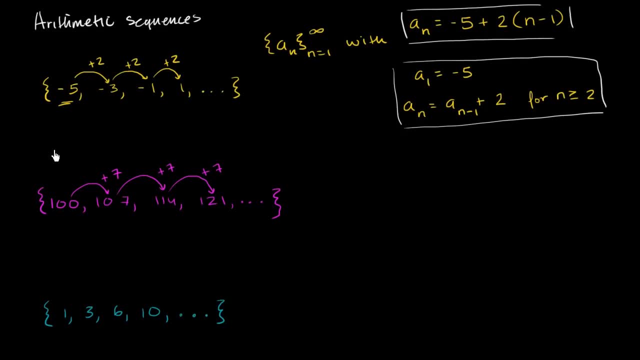 We are adding 7. So this is indeed an arithmetic sequence, just to be clear. This is 1. And this is 1 right over here. 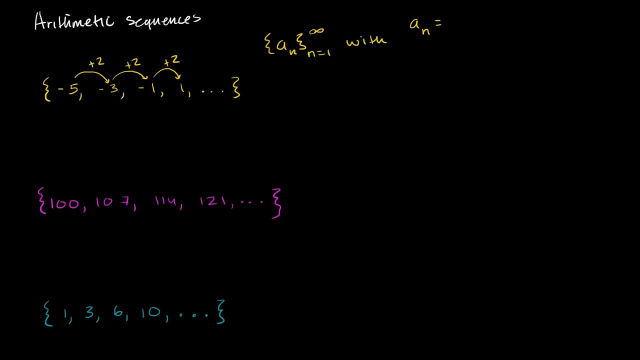 Is equal to whatever the first term is. In this case, our first term is negative 5.. It's equal to negative 5 plus we're going to add 2 one less times than the term we're at. So for the second term, we add 2 once. 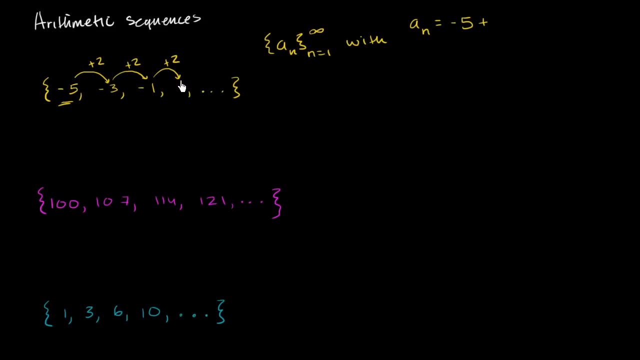 For the third term, we add 2 twice. For the fourth term, we added from our base term. we added 2 three times. So we're going to add 2.. We're going to add positive 2.. 1 less than the index that we're looking at. 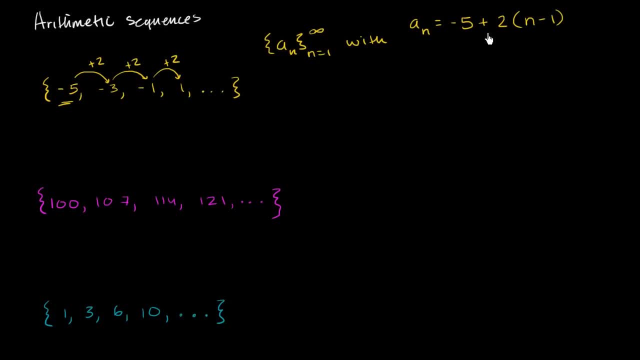 n minus 2.. Minus 1 times. So this is an explicit definition of this arithmetic sequence. If I wanted to write it recursively, I could say: a sub 1 is equal to negative 5. And then each successive term for a sub 2 and greater. 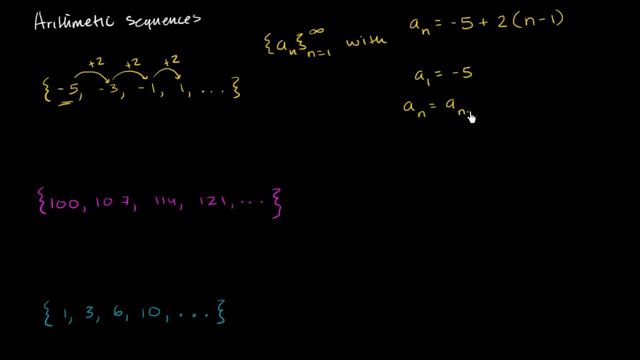 So I could say a sub n is equal to a sub n minus 1 plus 3.. Each term is equal to the previous term plus 2. Not 3.. So this is for For n greater than or equal to 2.. 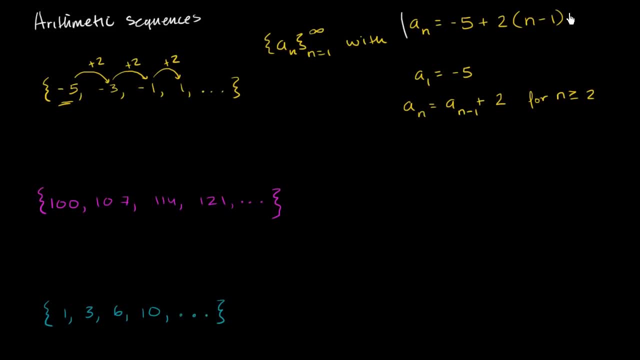 So either of these are completely legitimate ways of defining the arithmetic sequence that we have here. We could either define it explicitly or we could define it recursively. Now let's look at this sequence. Is this one arithmetic? Well, we're going from 100.. 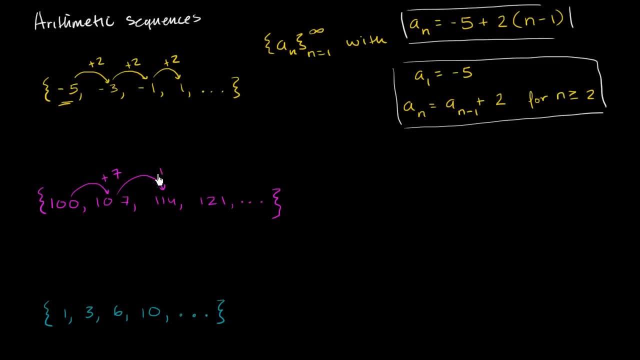 We add 7.. 107 to 114,. we're adding 7.. 114 to 121.. 121. We are adding 7.. So this is indeed an arithmetic sequence. just to be clear, This is 1. And this is 1 right over here. 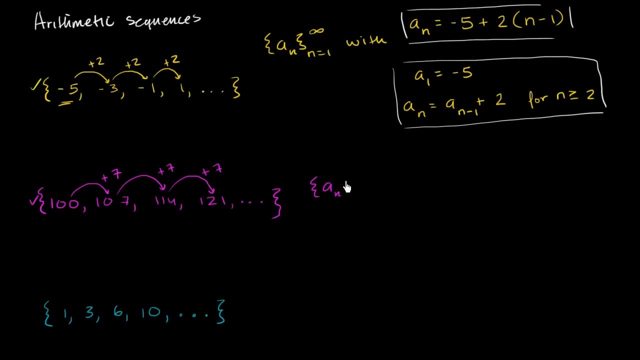 And we could write that. this is the sequence: a sub n? n going from 1 to infinity of- And we could just say a sub n, if we wanted to find it explicitly- is equal to 100 plus we're adding 7 every time. 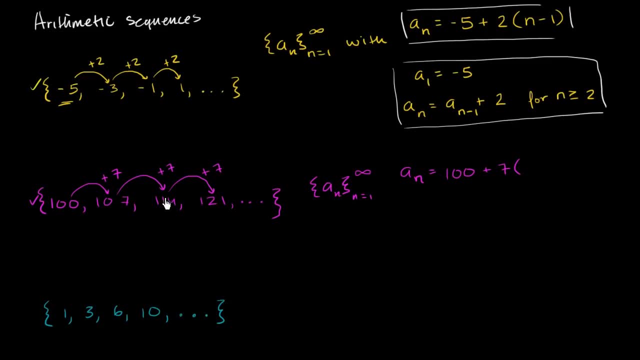 And then each term. the second term, we added 7 once. The third term, we add 7 twice. So for the n-th term, we're going to add 7 n minus 1 times. So this is an explicit definition of it. 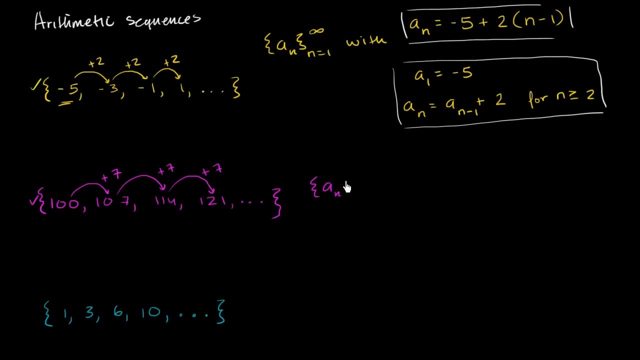 And we could write that this is the sequence a sub n, n going from 1 to infinity of. And we could just say a sub n, if we wanted to find it explicitly, is equal to 100 plus we're adding 7 every time. 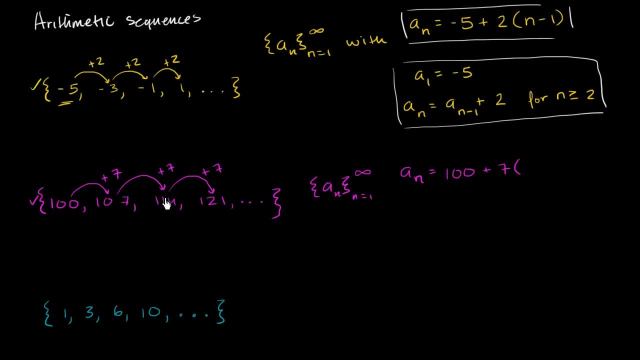 And then each term, the second term we added 7 once. The third term we add 7 twice. So for the n-th term, we're going to add 7 n minus 1 times. 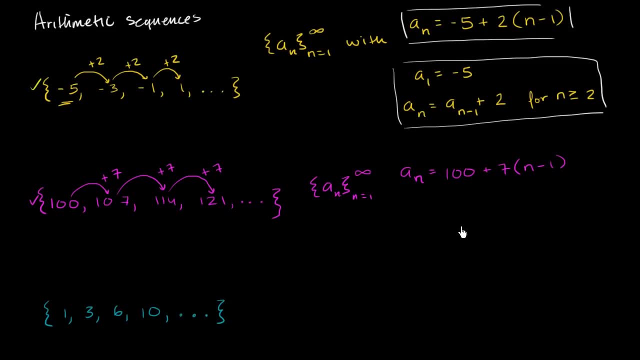 So this is an explicit definition of it. But we could also do it recursively. 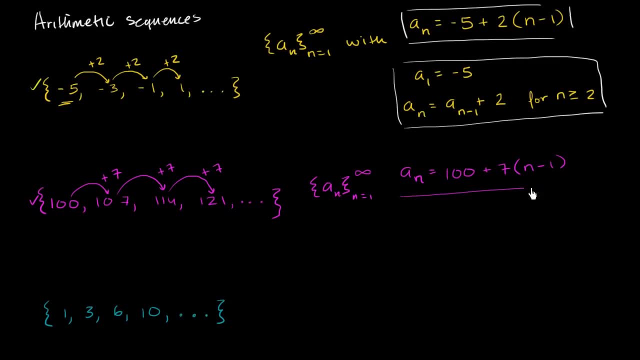 We could also say, we could also, so just to be clear, this is one definition where we write it like this. Or we could write a sub n from n equals 1 to infinity. In either case, I should write with. 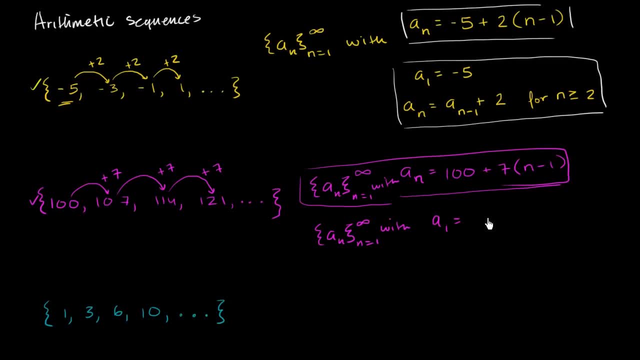 And if I wanted to find it recursively, I could say, a sub n. A sub 1 is equal to 100. And then for a sub n, for anything larger than 1, for any index above 1, a sub n is equal to the previous term plus 7. And so we're done. 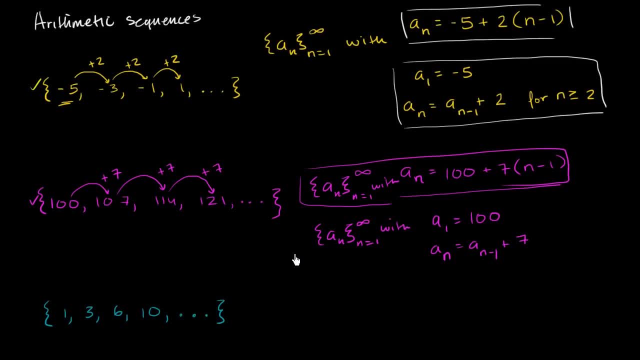 This is another way of defining it. So in general, if you wanted a generalizable way 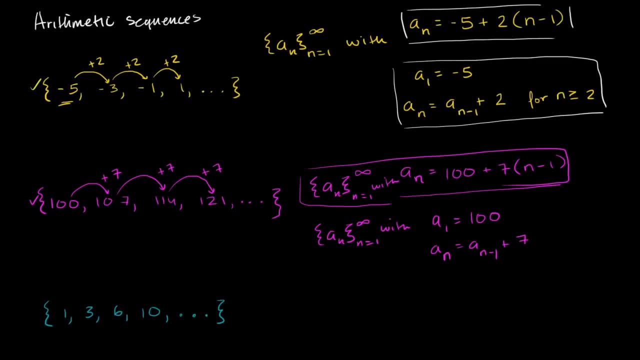 to spot or define an arithmetic sequence, you could say an arithmetic sequence is going to be of the form a sub n, if we're talking about an infinite one, from n equals 1 to infinity. 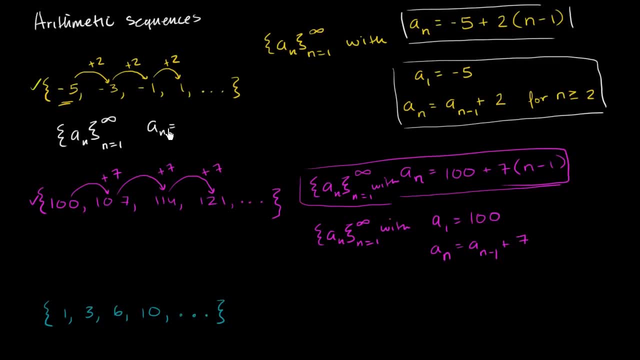 If you wanted to find it explicitly, you could say a sub n is equal to some constant, which would essentially be the first term. It would be some constant plus some number that you're incrementing, or I guess this could be a negative number, or decrementing by, times n minus 1. So this is one way to define an arithmetic sequence. 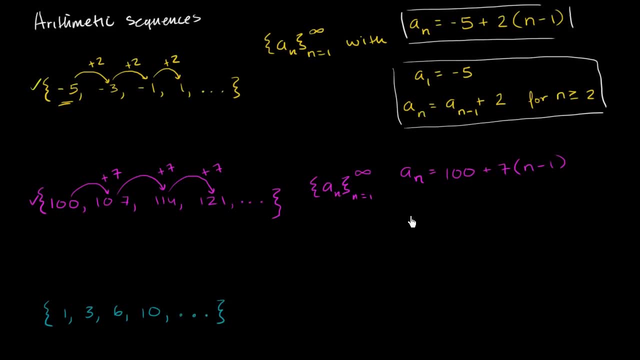 But we could also do it recursively. We could also say: we could also. so just to be clear, this is one definition where we write it like this: Or we could write a sub n from n equals 1 to infinity. In either case, I should write with: 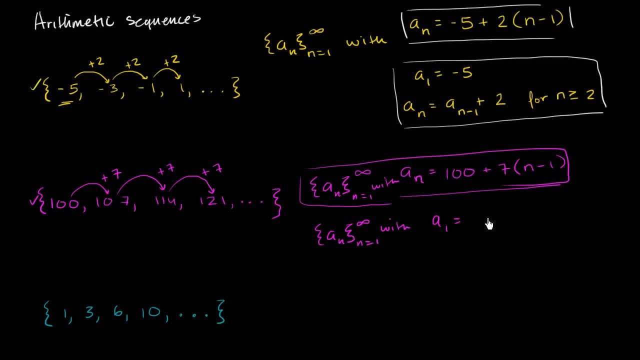 And if I wanted to find it recursively, I could say: a sub n, A sub 1, is equal to 100.. And then for a sub n for anything larger than 1, for any index above 1, a sub n is: 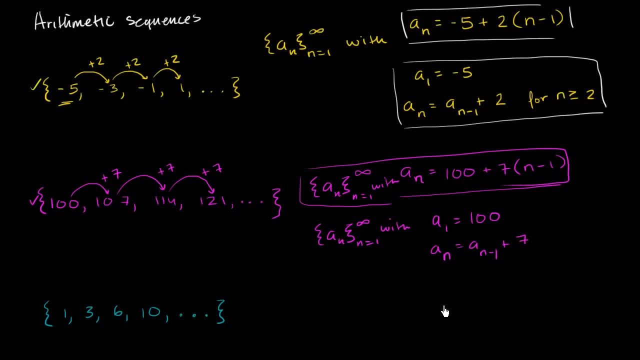 equal to the previous term plus 7.. And so we're done. This is another way of defining it. So, in general, if you wanted a generalizable way to spot or define an arithmetic sequence, you could say: an arithmetic sequence is going to be of the form a, sub n. 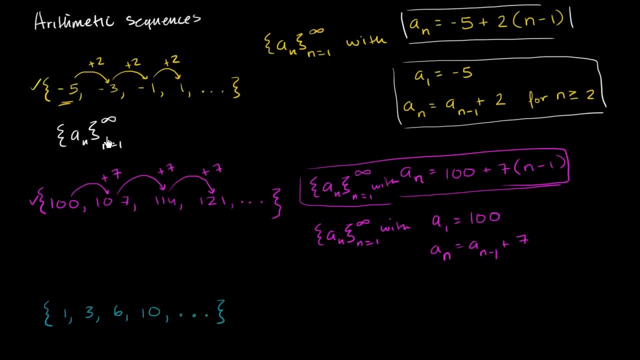 if we're talking about an infinite one, from n equals 1 to infinity. If you wanted to find it explicitly, you could say: a sub n is equal to some constant, which would essentially be the first term. It would be some constant plus some number. 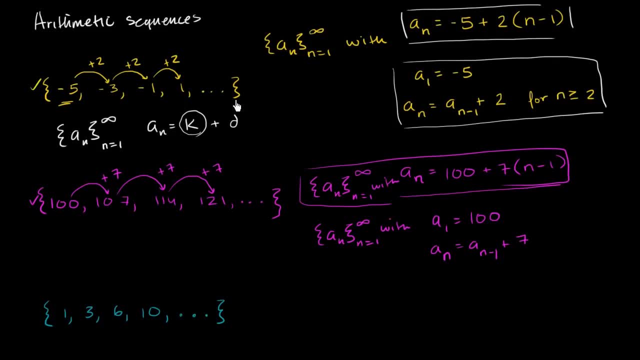 that you're incrementing- or I guess this could be a negative number- or decrementing by times n minus 1.. So this is one way to define an arithmetic sequence. In this case, d was 2.. In this case, d is 7.. 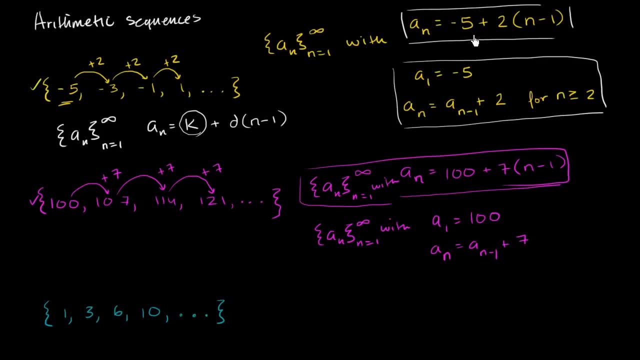 That's how much you're adding by each time, And in this case k is negative 5.. And in this case k is 100.. The other way that you could, if you wanted to write the recursive way of defining an arithmetic sequence generally: 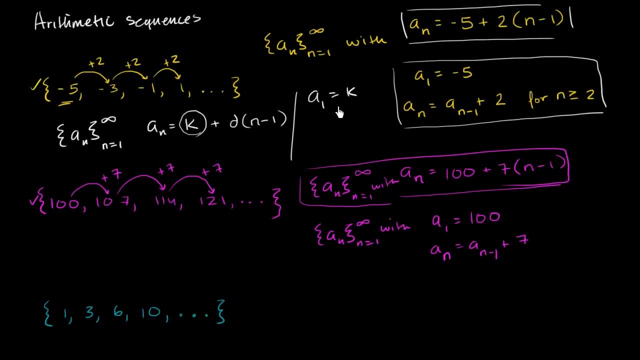 you could say: a sub 1 is equal to k And then a sub n is equal to a sub n minus 1.. A given term is equal to the previous term plus d for n greater than or equal to 2.. So once again, this is explicit. 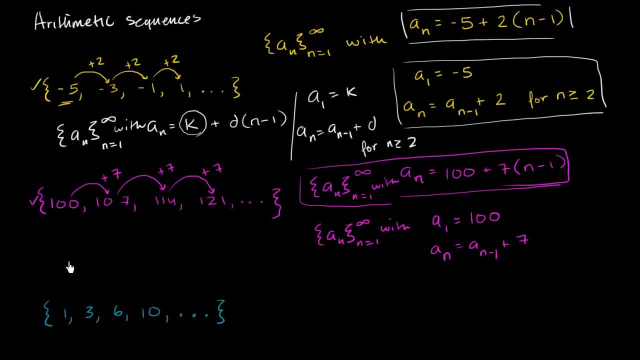 This is the recursive way, This is the way of defining it, And we would just write with there. Now, the last question I have is: is this one right over here an arithmetic sequence? Well, let's check it out. To start, we start at 1.. 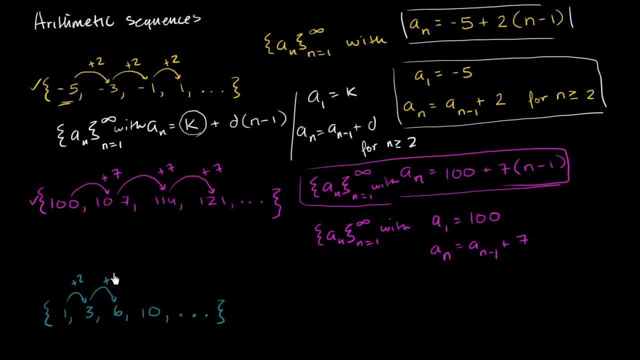 Then we add 2.. Then we add 3.. So this is an immediate giveaway that this is not an arithmetic sequence. Now we are adding 4.. We're adding a different amount every time, So this, first of all, this is not arithmetic. 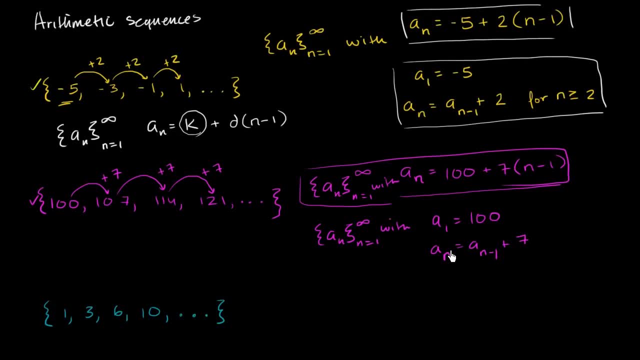 The other way that you could, if you wanted to write the recursive way of defining an arithmetic sequence generally, you could say a sub 1 is equal to k. 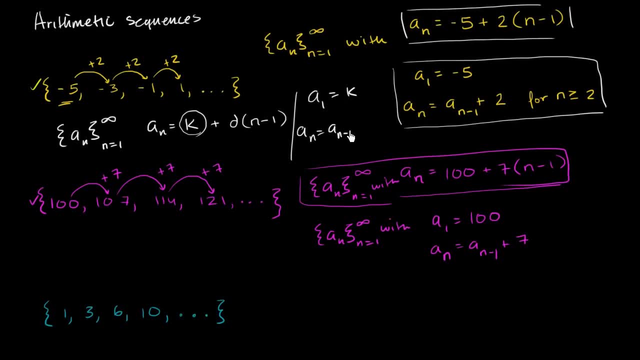 And then a sub n is equal to a sub n minus 1. A given term is equal to the previous term plus d for n greater than or equal to 2. 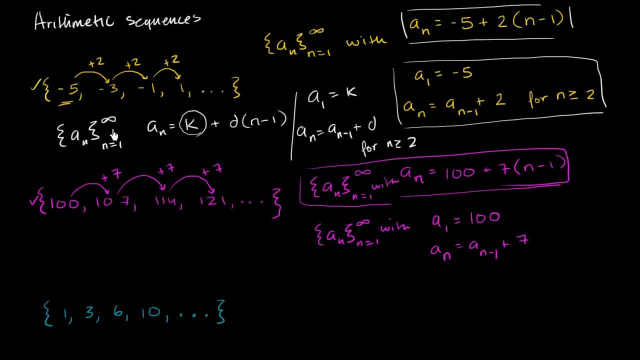 So once again, this is explicit. This is the recursive way of defining it. And we would just write with there. 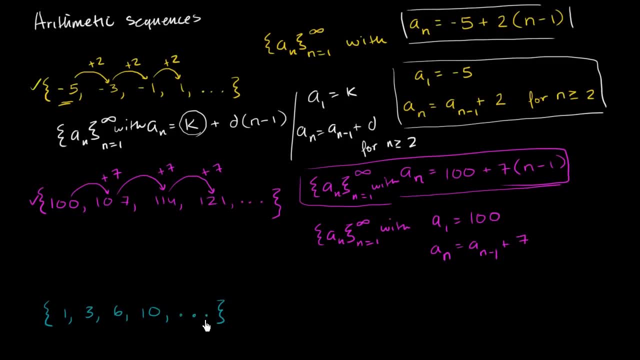 Now the last question I have is, is this one right over here an arithmetic sequence? Well, let's check it out. 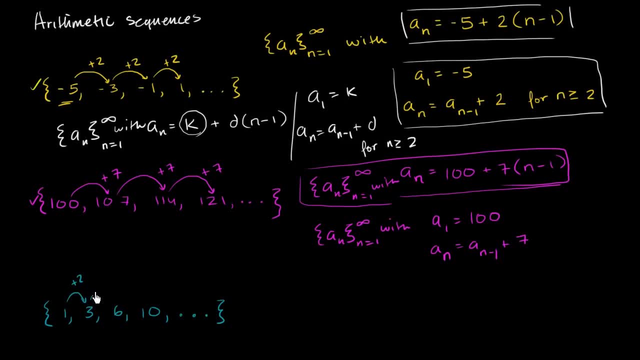 To start, we start at 1. Then we add 2. Then we add 3. So this is an immediate giveaway that this is not an arithmetic sequence. 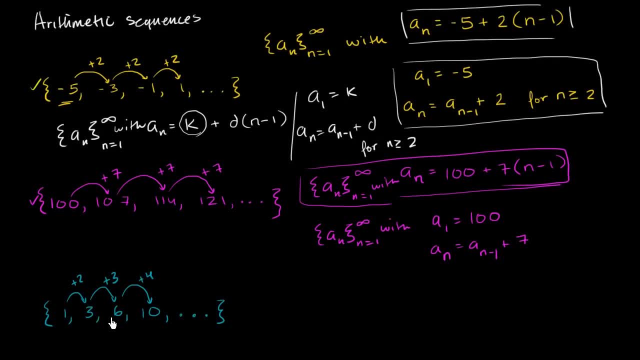 Now we are adding 4. We're adding a different amount every time. 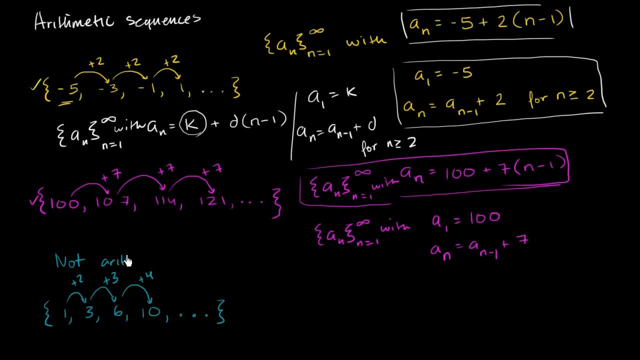 So this, first of all, this is not an arithmetic sequence. But how could we define this, since we're trying to define our sequences? So if we wanted to define it, let's say we wanted to define it recursively. 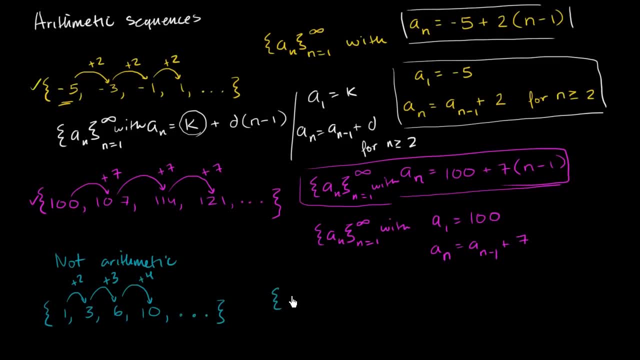 So we could say this is equal to a sub n, where n is starting at 1 and it's going to infinity, with, we'll say our base case, a sub 1 is equal to 1. And then for n is 2 or greater, a sub n is going to be equal to what? So a sub 2 is the previous term plus 2. a sub 3 is the previous term plus 3. a sub 4 is the previous term plus 4. So it's going to be the previous term plus whatever your index is. 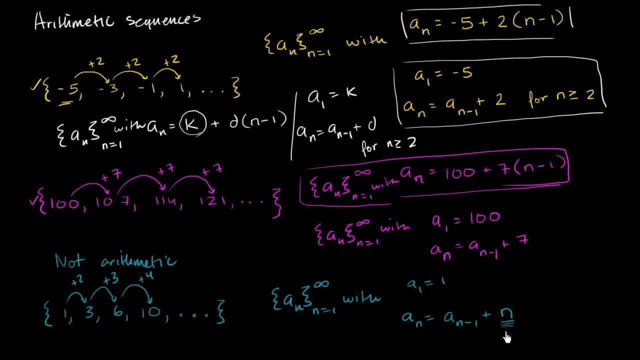 So this looks close, but notice, here we're changing the amount that we're adding based on what our index is. 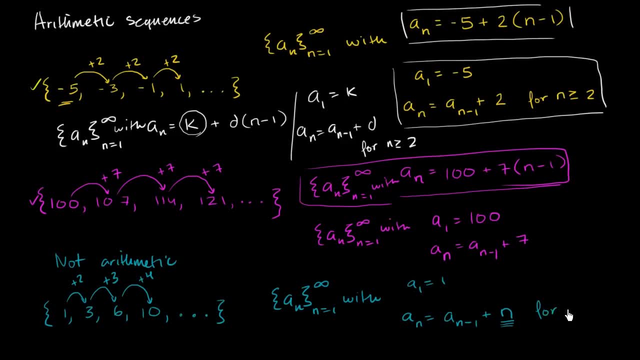 We're adding the amount of index to the previous term. And so this is 4. n is greater than or equal to 2. Well, for an arithmetic sequence, we're adding the same number of indexes. We're adding the same amount regardless of what our index is. 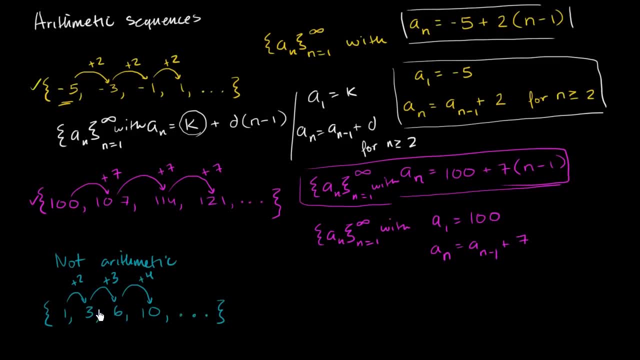 This is not an arithmetic sequence, But how could we define this, Since we're trying to define our sequences? So if we wanted to define it, let's say we wanted to define it recursively, So we could say: this is equal to a sub n, where 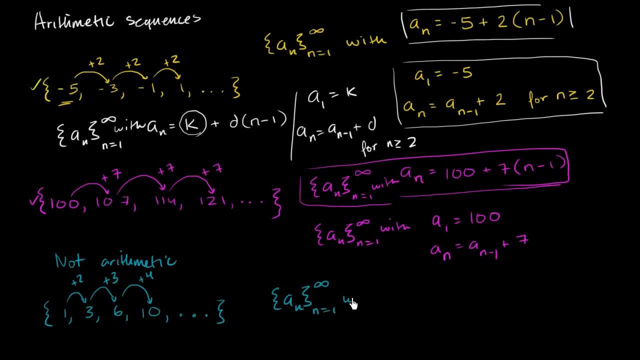 n is starting at 1 and it's going to infinity with, we'll say, our base case: a sub 1 is equal to 1.. And then, for n is 2 or greater, a sub n is going to be equal to what? 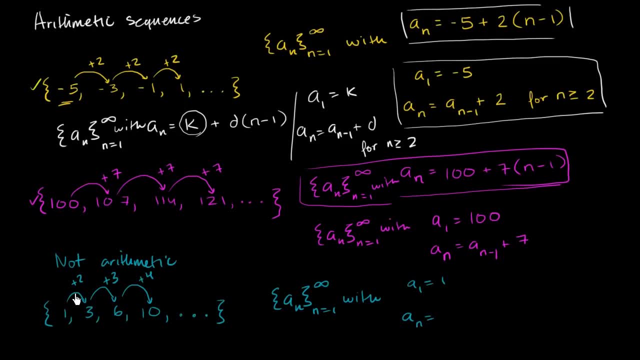 So a sub 2 is the previous term plus 2.. a sub 3 is the previous term plus 3.. a sub 4 is the previous term plus 4.. So it's going to be the previous term plus whatever your index is. 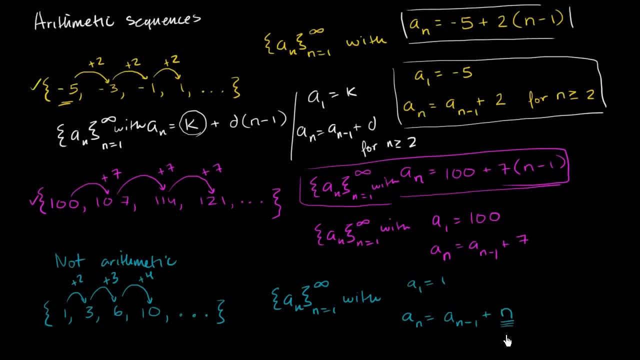 So this looks close. but notice, here we're changing the amount that we're adding based on what our index is. We're adding the amount of index to the previous term, And so this is 4.. n is greater than or equal to 2.. 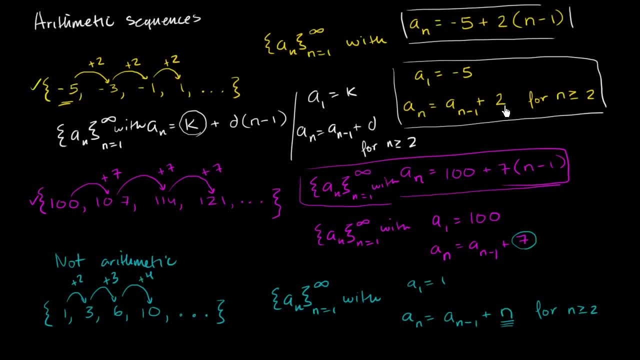 Well, for an arithmetic sequence, we're adding the same amount, regardless of what our index is. Here we're adding the index itself. So this one is not arithmetic, but it's an interesting sequence nonetheless. 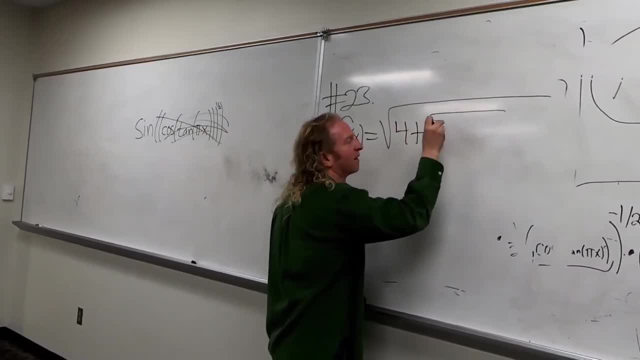 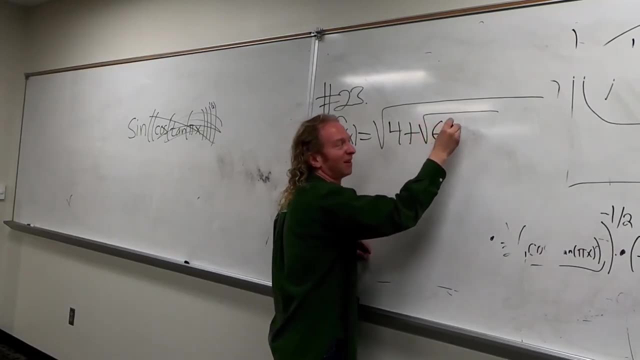 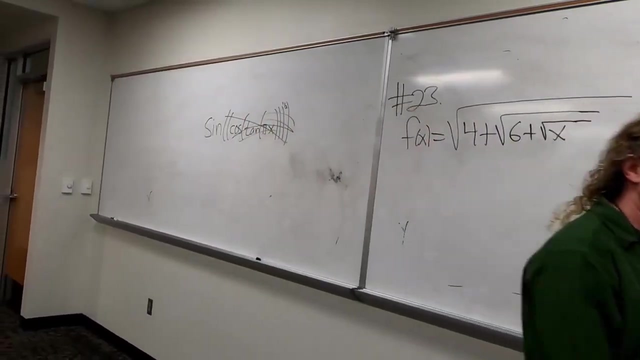 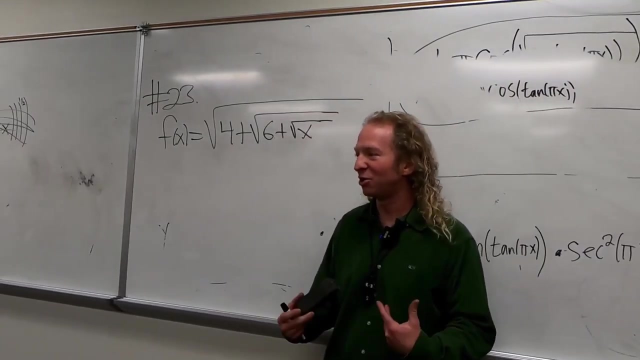 Like this: That's it, That's the problem. Okay, All right, Fun times. Okay. So do y'all want to try it, or should I just do it? We have six minutes Just to be. you want to try it? Try it, Try it. Take two minutes, Two minutes, Go Try it, Try it.